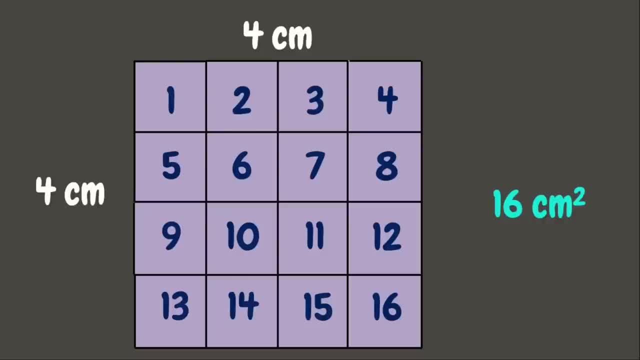 centimeters squared, It means that its area is 16 square centimeters. Now here we can observe that if we multiply 4 cm by 4 cm, We will get the area which is 16 square centimeters. It means that the formula to get the area of a square is: 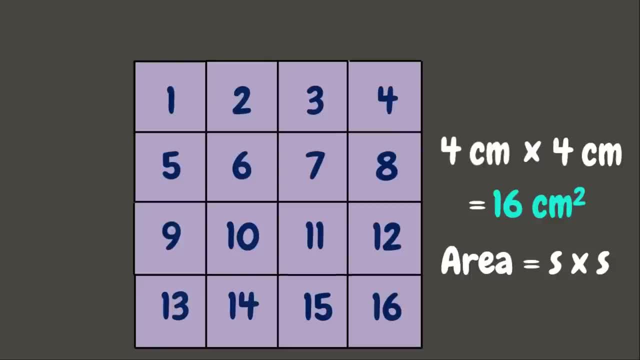 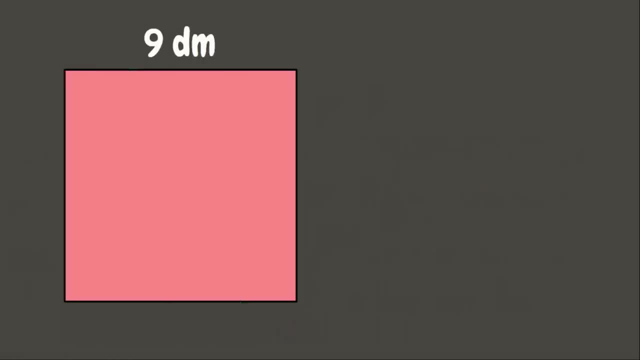 Side times side or S times S or S squared. Now let's try this formula To our next example. Again, we have your square, But this time each side measures 9 decimeters. Again, the formula for the area of square is Side times side or S squared. 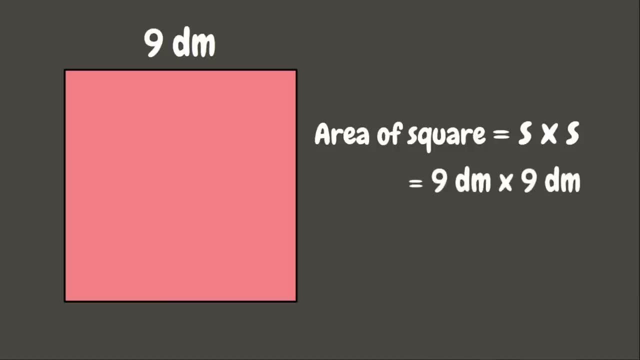 So here the measure of the side is 9 decimeters, So that will be 9 decimeters times 9 decimeters. If we multiply that, that will be 81 square decimeters And that is the area of this square. Wonderful, Now let's go and have another example. 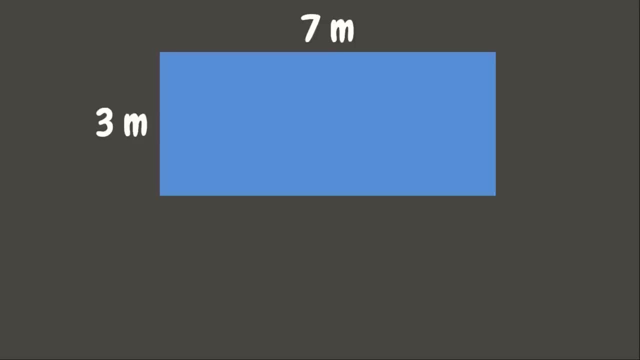 This time we have our rectangle, Whose length measures 7 meters. It means that it has 7: 1 meters. Now let us count 1,, 2,, 3,, 4,, 5,, 6, and 7, While its width measures 3 meters. 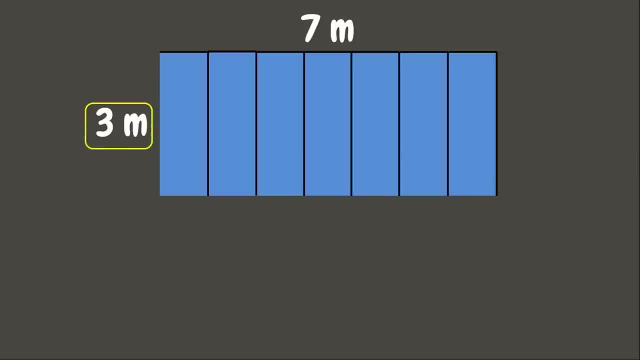 It means that it has 3, 1 meters. So let's count 1,, 2,, 3,, 4,, 5,, 6, and 7 And 3. Now we already have some square units Now to get its area. 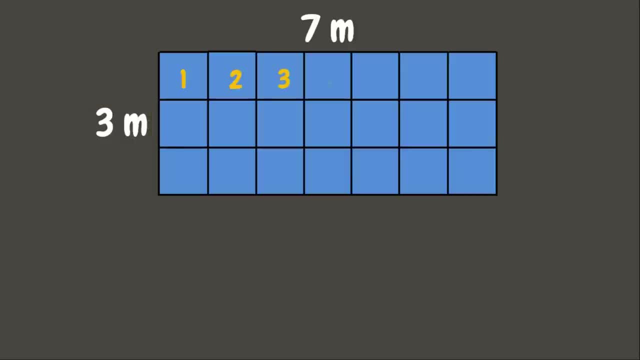 Let us count them Now. we have 21 square meters And that is its area. Now we can observe that If we multiply 7 meters to 3 meters, We will get its area, which is 21 square meters. It means that if we multiply 7 meters to 3 meters, 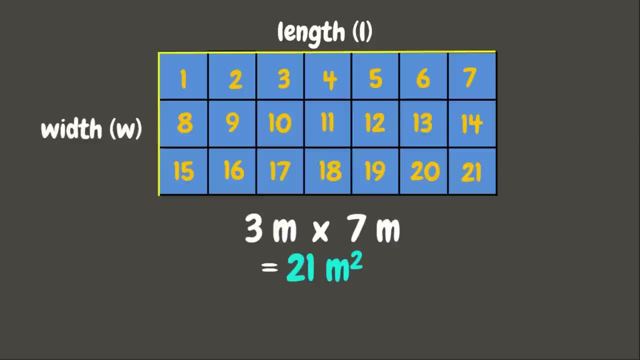 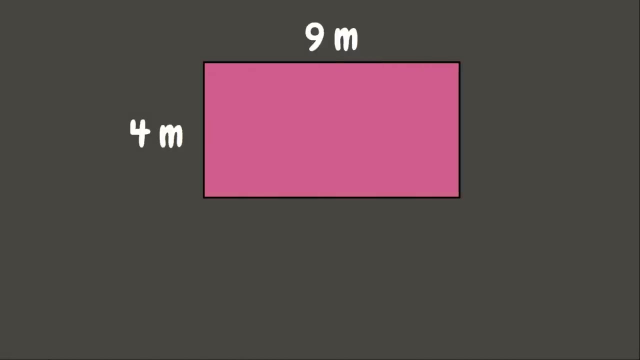 If we multiply the length and the width, We are going to get its area. Therefore, the formula for the area of rectangle is Length times width. Now let's try this formula for our next example. Again, we have here a rectangle Whose length measures 9 meters. 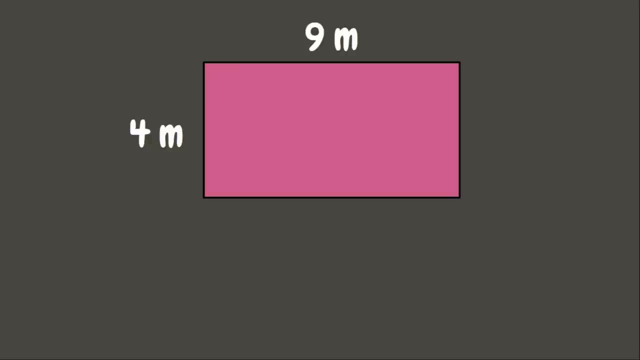 And width measures 4 meters. Now let us solve. We have the formula for the area of rectangle, Which is length times width. Now let's multiply 9 meters to 4 meters, And that will be 36 square meters. Great job. Now we have here another example. 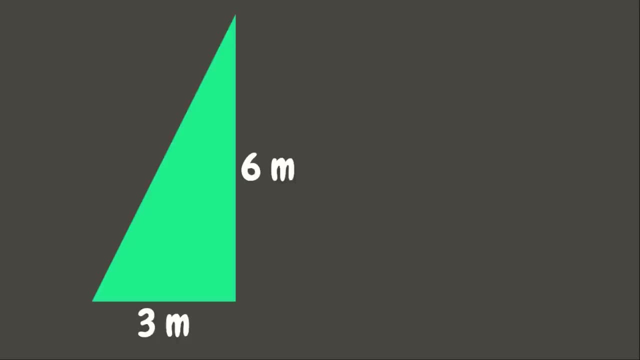 This time we have a triangle Whose one side measures 6 meters, So that means it has 6: 1 meters. So let us count 1,, 2,, 3,, 4,, 5, and 6, While the other side measures 3 meters. 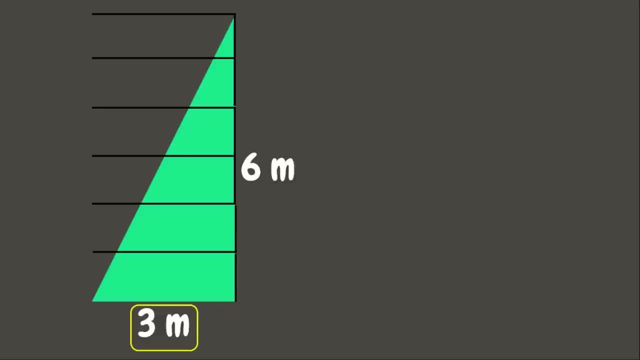 It means that it has 3: 1 meters. Now let us count 1,, 2, and 3. Now, if we count the number of square units That we have here, That will be 18 square meters, But we can see that we form a rectangle. 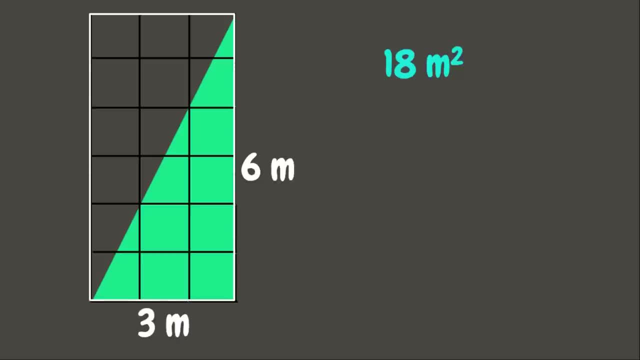 So that means that we have 18 square meters, But we can see that we form a rectangle And 18 square meters is the area of the rectangle form. But we are only looking for the area of the triangle. As we can observe, The triangle is the half of the rectangle. 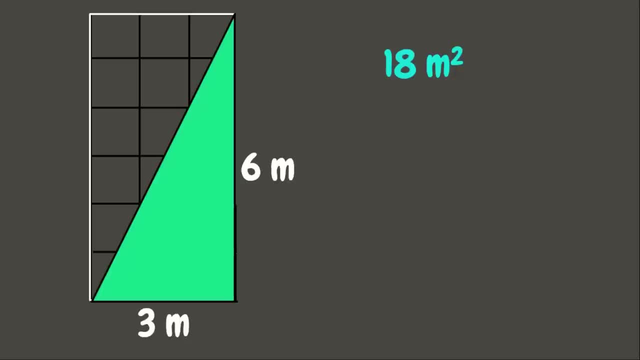 It means that if we divide our area, Which is 18 square meters, into 2, That would be 9 square meters, Which is the area of the triangle. We can observe, If we multiply them- back and forth measures of each side, which is 3 meters and 6 meters, and divided to 2, we will get the area. 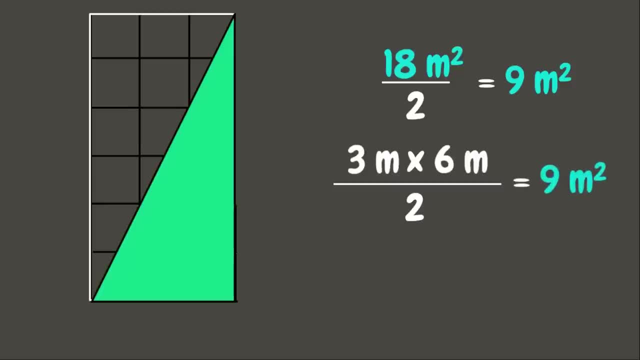 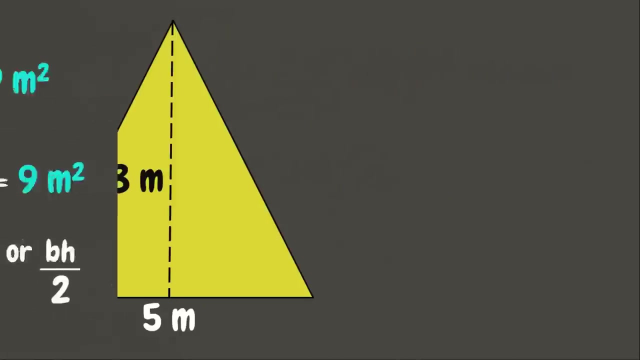 of the triangle, which is 9 square meters. therefore, the formula for the area of triangle would be base times the height divided by 2, or b times h divided by 2. now let's try this formula and solve another example. here we have another triangle whose. 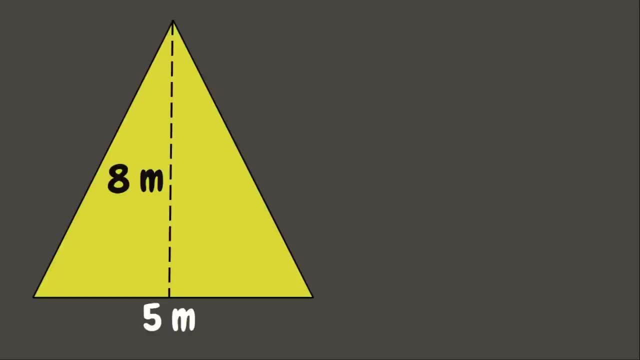 height measures 8 meters, while the base measures 5 meters again. the formula for the triangle is base times height divided by 2.. now let us solve. we have 5 meters times 8 meters divided by 2.. 5 meters times 8 meters. 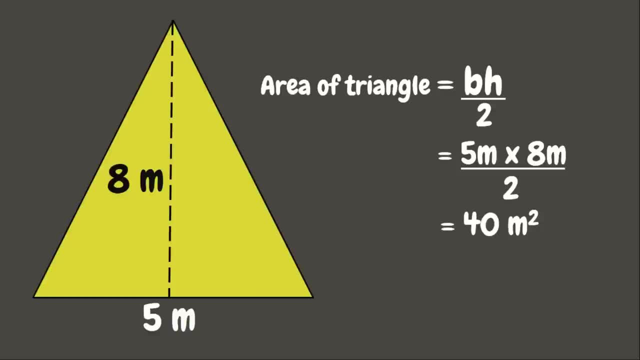 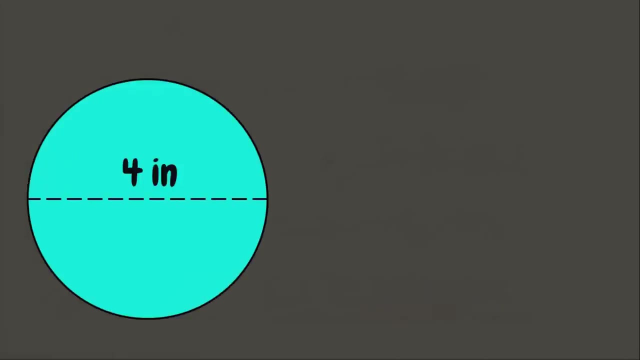 is great job. it's 40 square meters. now let's divide it into two and that will be 20 square meters, and that is the area of the triangle. wonderful, now let's have another example. this time we have a circle. to get the area of a circle, we 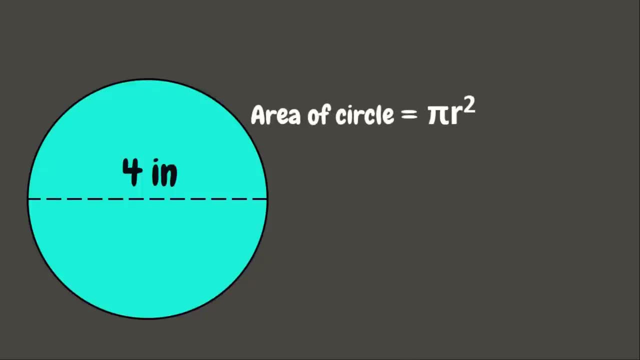 are going to use the formula PI, R squared. here the volume file we are going to use is 3.14. now the R stands for radius. their radius is the half of the diameter, which is the 4 inches. therefore, the half of the diameter, which is 4 inches, is 2 inches. but here we need to get a squared of the. 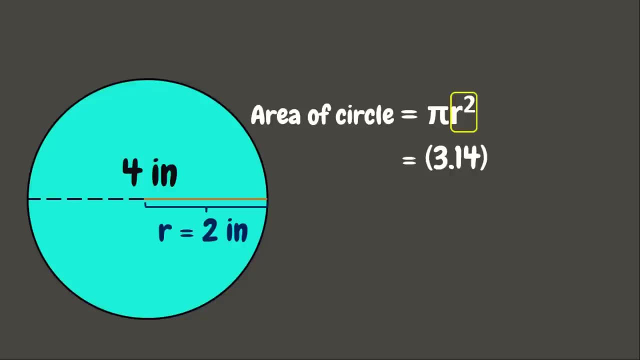 radius. this means that we are going to multiply it by itself two times, so that will be 2 inches times 2 inches. now let us solve: 2 inches times 2 inches is 4 square inches. now let's multiply 3.14 by 4 square inches and that will be 12.56. 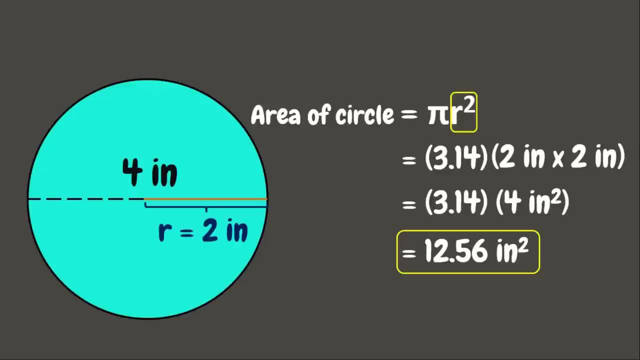 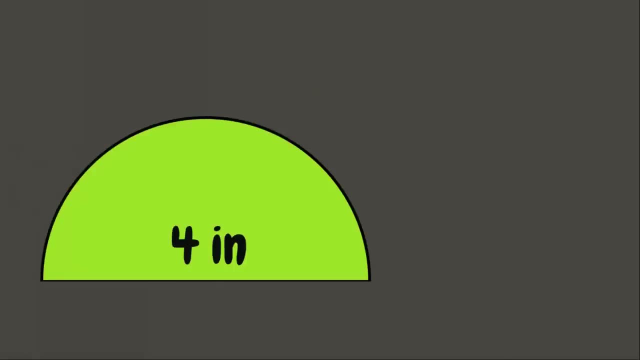 square inches and that is the area of this circle. correct me if I'm wrong, great job. now let's move on to our last example. this time we have a semicircle. a semicircle is half of a circle. now, to get the area of a semicircle, we just simply: 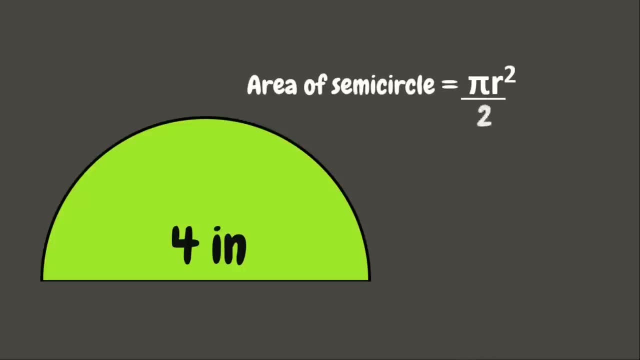 need to divide the PI R squared by 2 again. the volume file that we are going to use is 3.14 and the radius here is half of the diameter, which is 4 inches, and the halve of the 4 inch diameter, greater than 5 inch, is equal to the 2 right arrow line, if that someplace we saw theALKjęł. 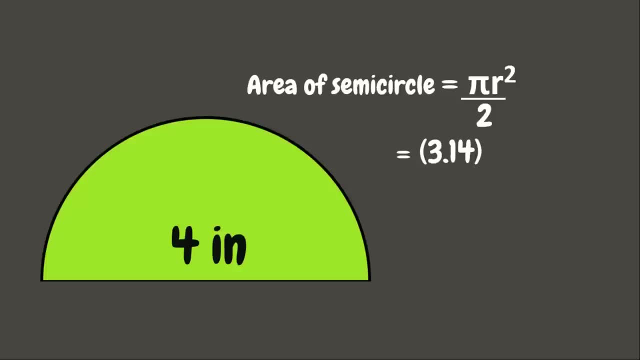 inches, and the half of the four inches is two inches, so that will be two inches times two inches divided by two. now let us solve. we have 12.56 square inches divided by two, and that would be 6.28 square inches, and that is the area of this semicircle. wonderful, you made it this far, students. now. here are the things that you learned today.